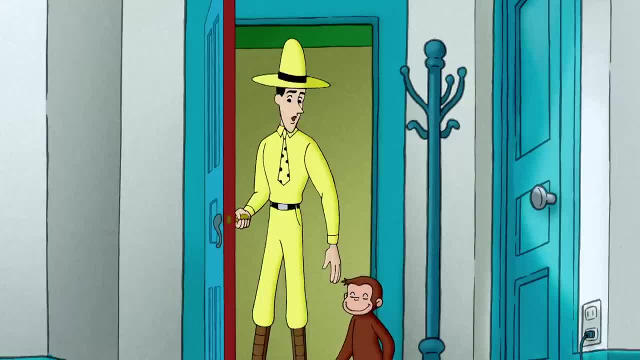 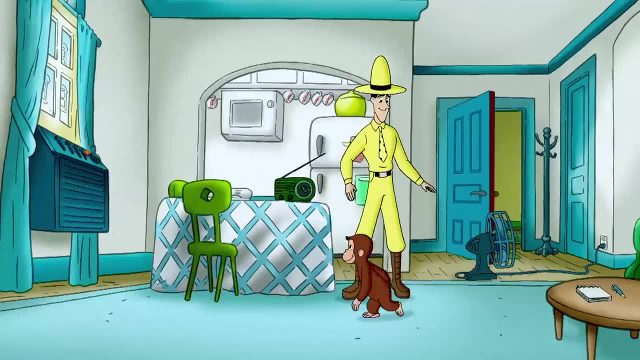 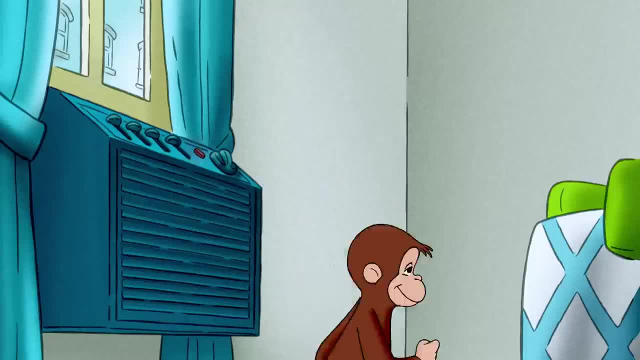 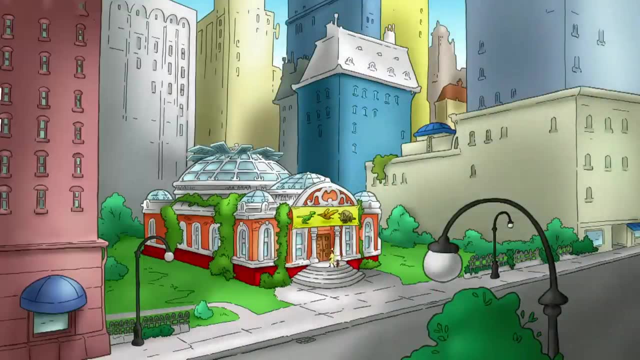 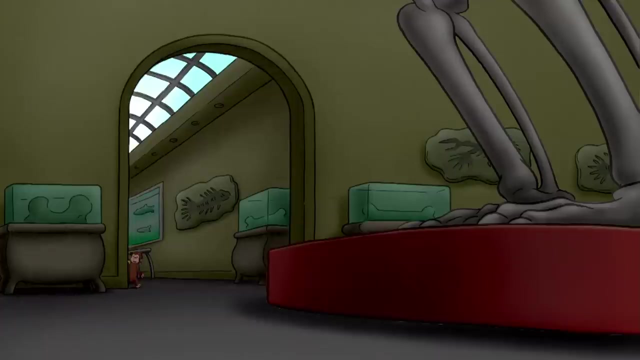 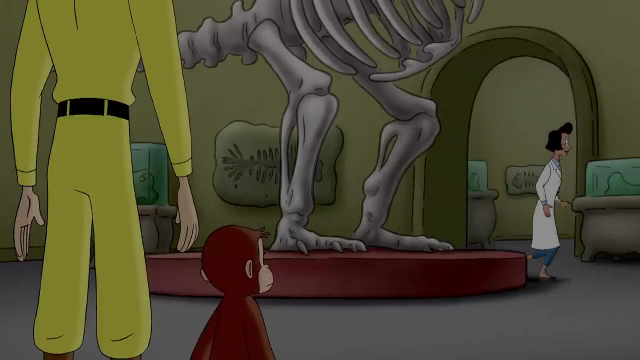 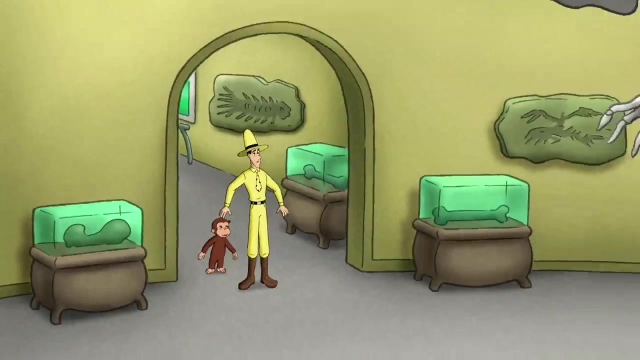 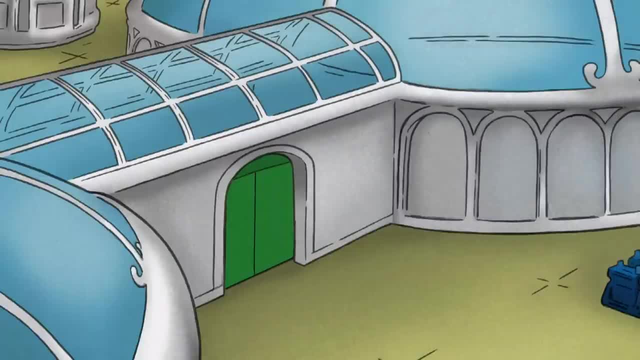 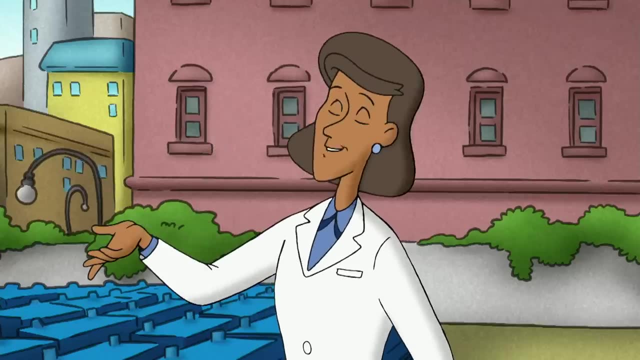 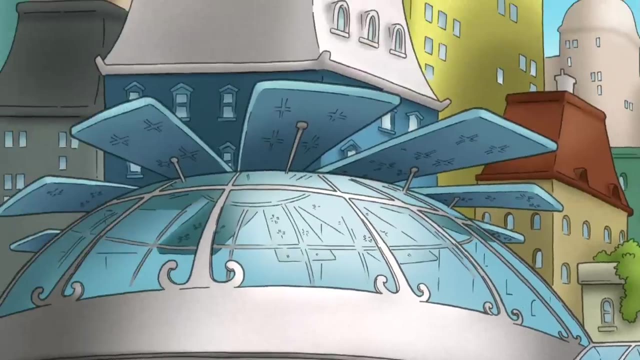 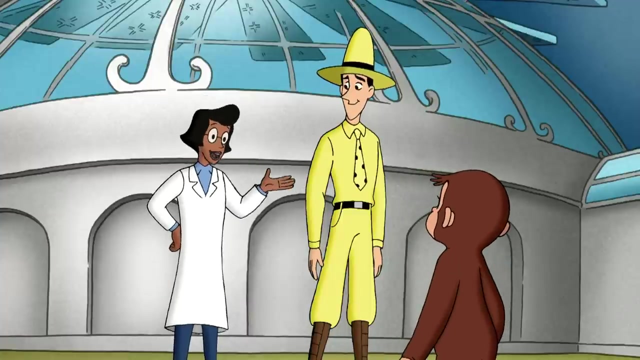 To see that the lights work. You just witnessed the first test of the solar panels I installed to power the museum. We're unveiling them at a party tonight. We're a solar museum, Wow. Usually electricity is made far away and sent in on wires, but now the museum makes its own power. 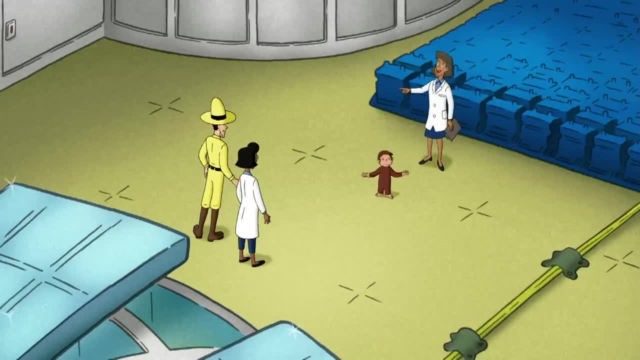 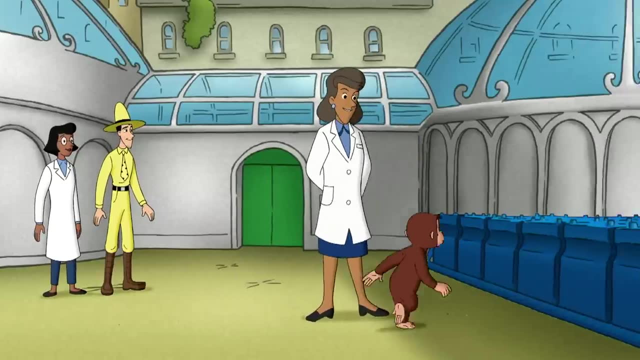 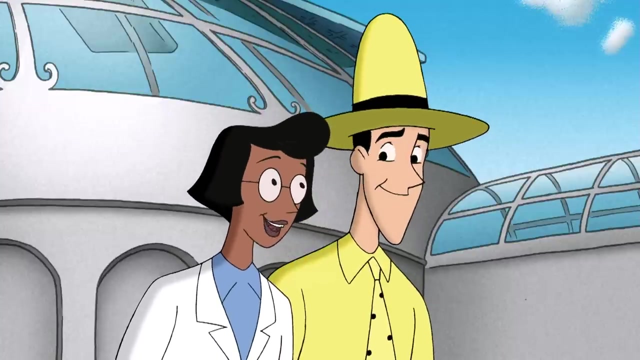 Solar panels turn the sun's rays into electricity, which is then stored in these batteries. It's Dr Levitt's birthday During the party for the solar panels. I'd like to give her a surprise. Oh, I could make one of my famous birthday lasagnas. 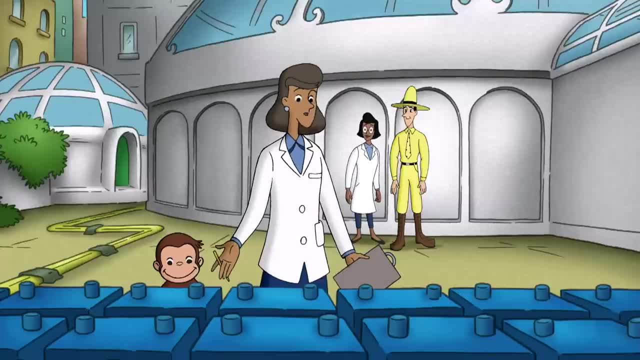 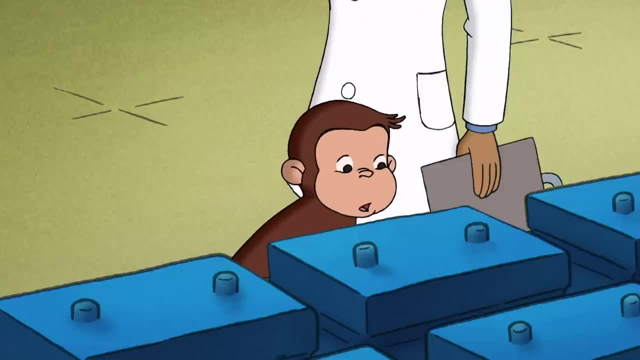 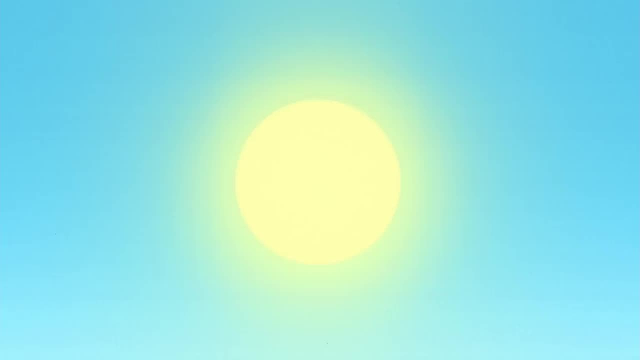 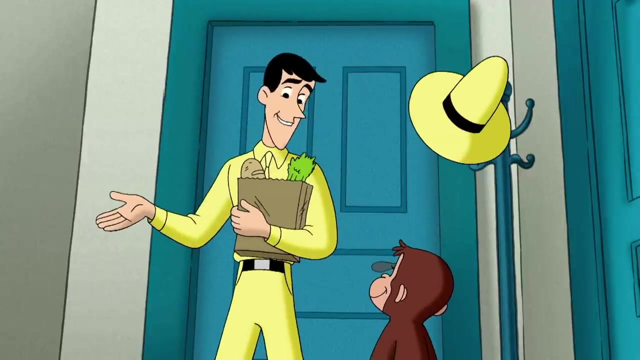 Precisely what I was thinking. These batteries are a lot like the ones in toys, flashlights or cordless phones, And they get all their power from the sun. George never knew the sun could charge batteries. I'm going to be busy with my lasagna so I can't play now, okay. 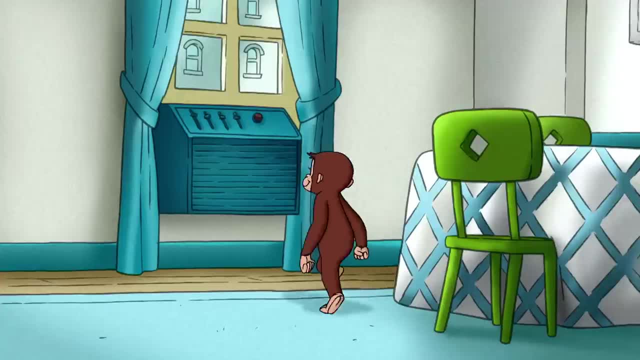 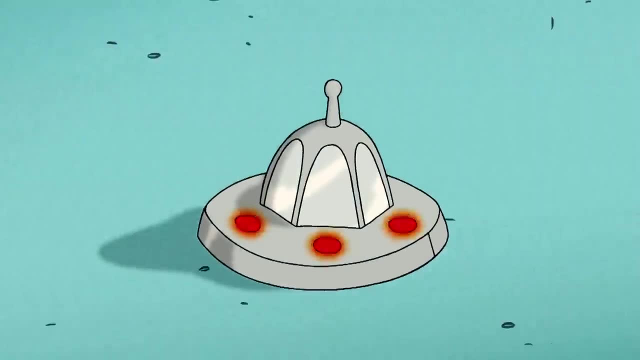 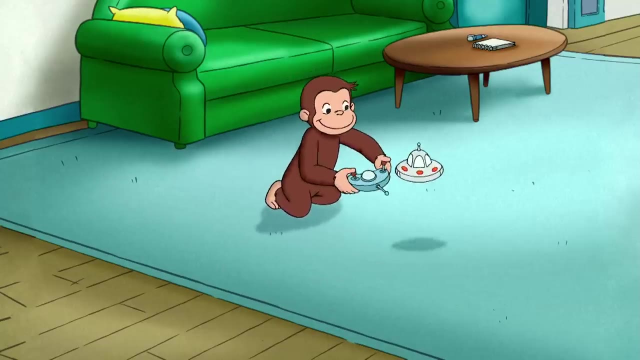 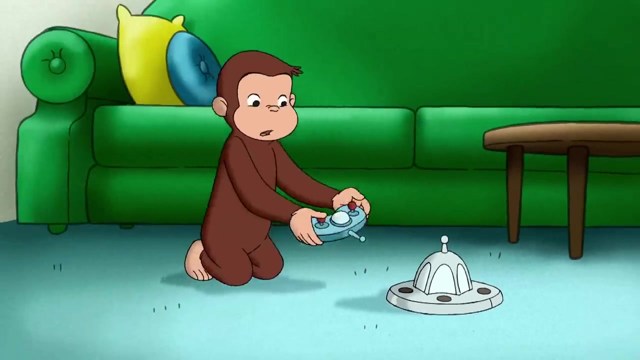 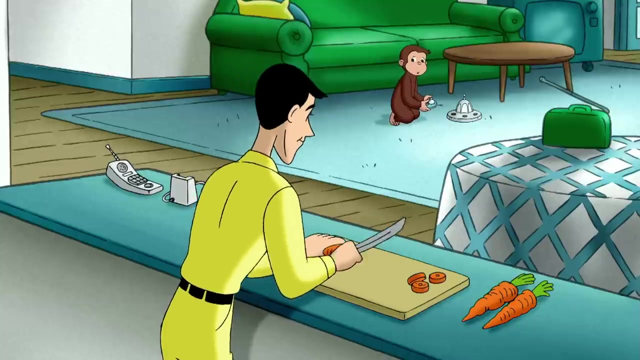 Okay, I'll be right back. A remote-controlled spaceship is the perfect hot-weather toy, Until the batteries run out. D'oh, I'm lost. George didn't want to bother the man with the yellow hat in mid-lasagna. 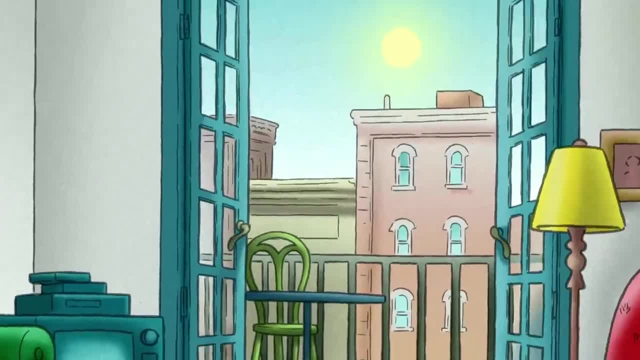 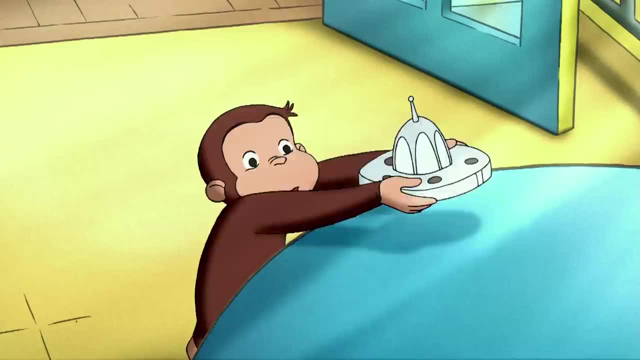 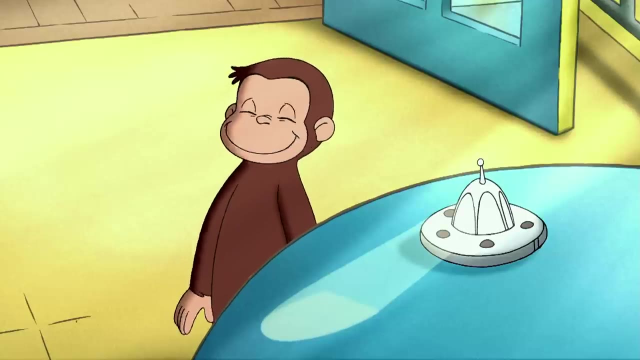 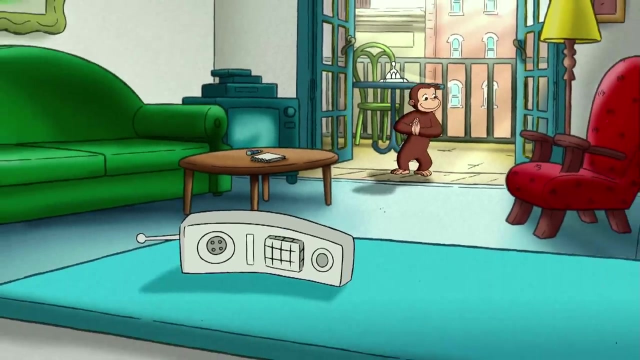 But he needed batteries. Then he remembered how the museum batteries got power from the sun. Ah, So why not let the sun charge up his batteries too? Ha-ha-ha, Ooh, Ooh, There was something else with batteries that needed charging. 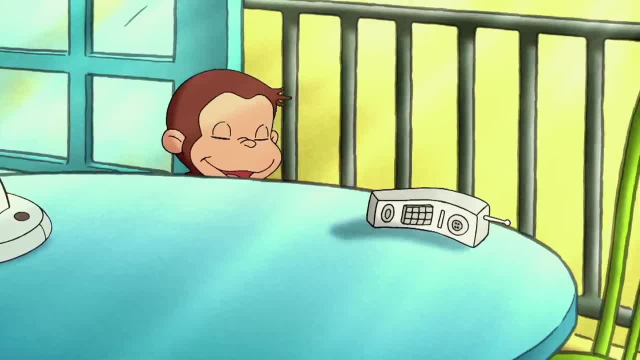 Ha-ha-ha, Ooh, Ha-ha-ha Ha, Ha-ha-ha, Ha, Ha-ha-ha Ha. 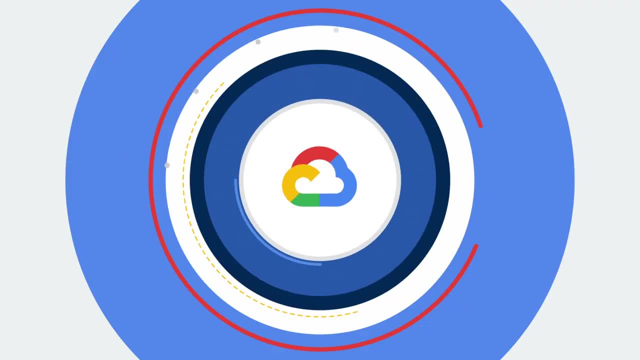 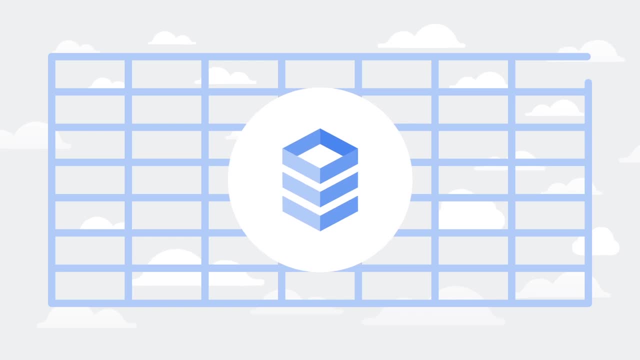 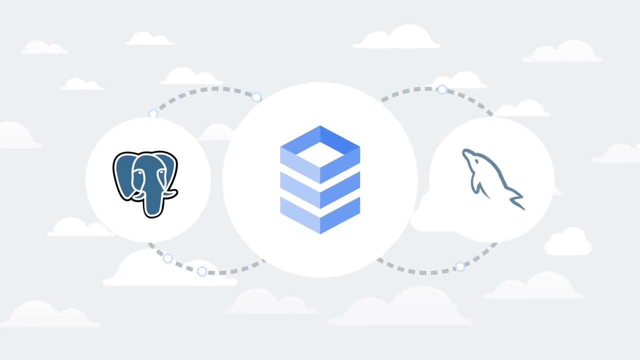 Give me one minute and I'll show you how Cloud SQL can help you save time in developing your next great app. Cloud SQL is a fully managed relational database service from MySQL, Postgres or SQL Server on Google Cloud. It lets you hand off mundane, time-consuming tasks like 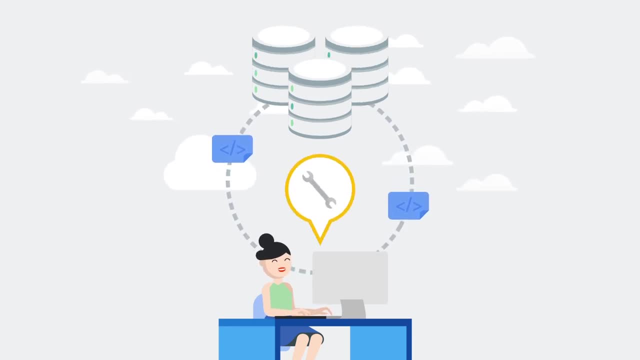 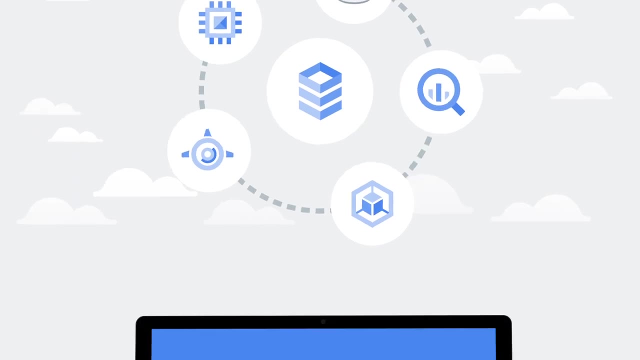 patches, updates, backups and replicas, so you can focus on building your app. Cloud SQL integrates with BigQuery for analytics or can act as a backend to your App Engine, Compute Engine or Kubernetes apps. Setting up Cloud SQL is quick and seamless: In a snap you can create an instance. 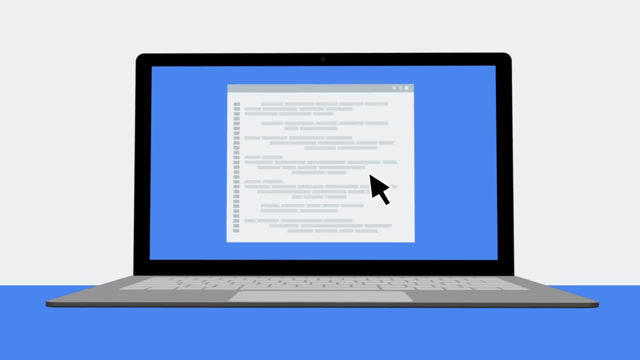 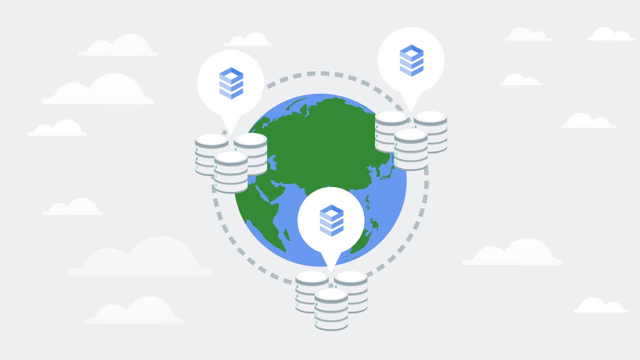 with the cloud console by choosing the type of database version and location, or use the gcloud command line, and then you're ready to upload your data or connect your applications. To go further, set up automatic backups, replication and failover, so you can create a highly available 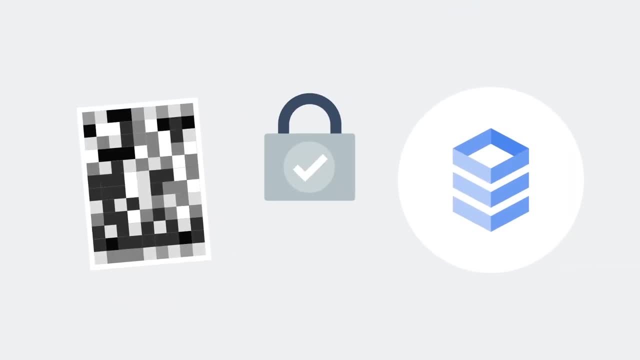 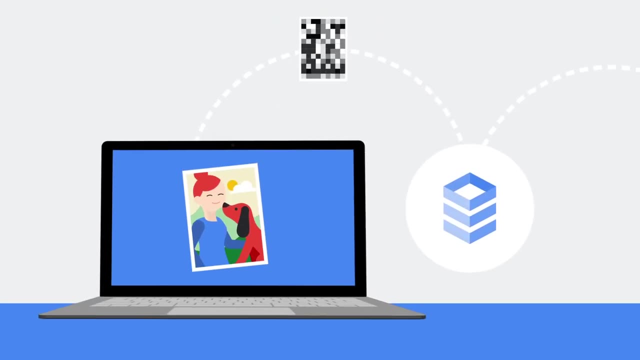 database for critical applications. You get full encryption at Reston and Transit, keeping your private data safe and compliant. External connections can be encrypted using SSL or Cloud SQL Proxy. Being a relational database, Cloud SQL is great for OLTP, where frequent queries and fast response times are needed. 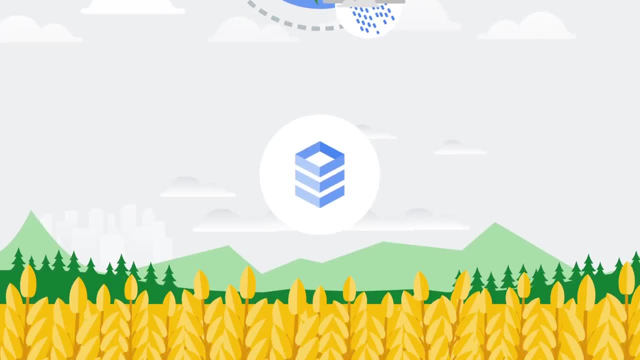 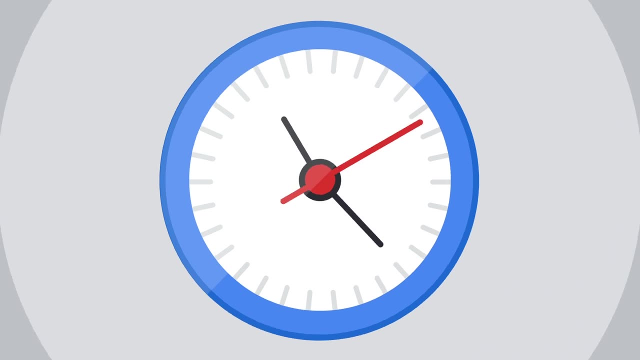 So you can use it to manage everything from a single WordPress blog to a global aggregation of wheat, crops and rainfall. Next time you're looking for a quick relational database solution, take a minute to try out Cloud SQL. To learn more, check out cloudgooglecom.